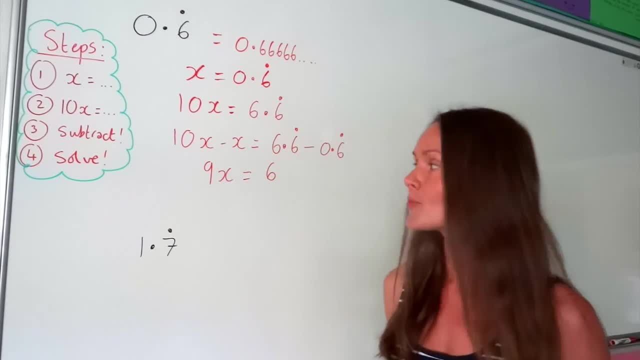 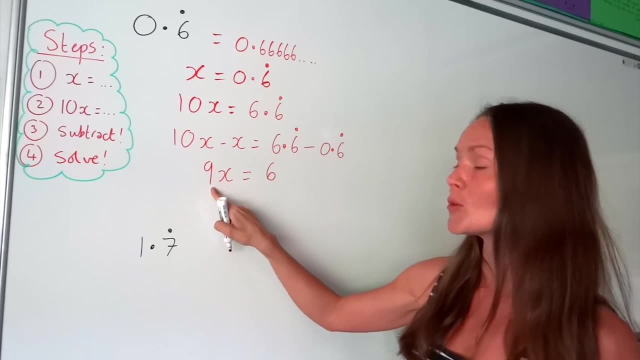 decimals here and I'm just left with the whole number 6.. So the last step is to solve this equation, to find x. So, because x is being multiplied by 9, the opposite is to divide by 9.. So I have to divide. 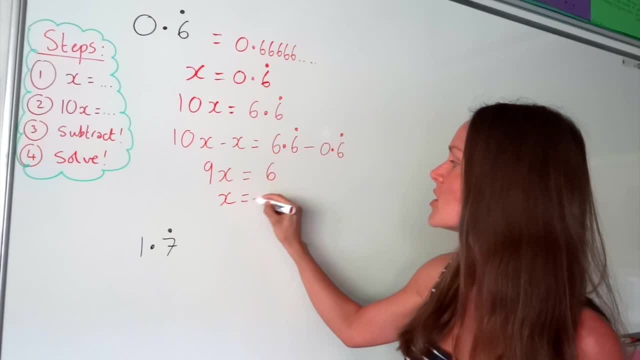 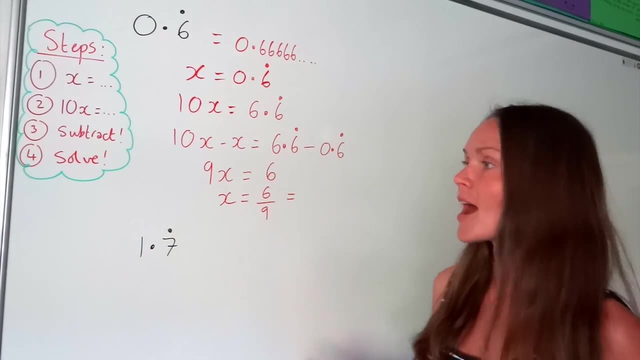 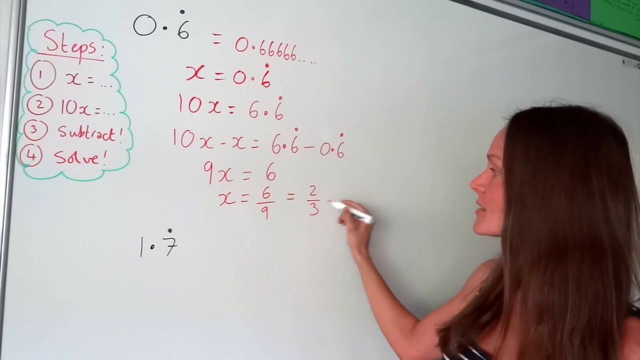 by 9 on both sides of the equation to keep it balanced. So I'm left with 6 over 9, which is our fraction. but we can simplify it because both of these numbers have a factor of 3.. So I can divide the top by 3 and the denominator by 3 as well. So there's our final fraction. 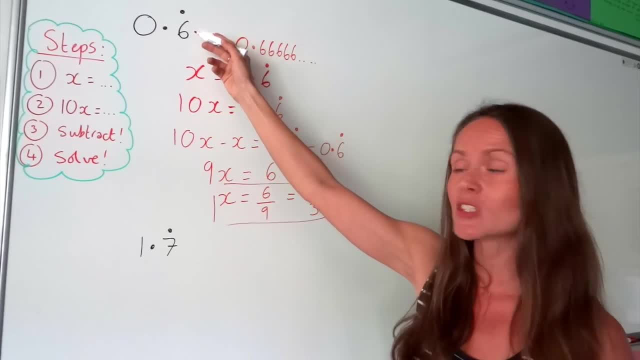 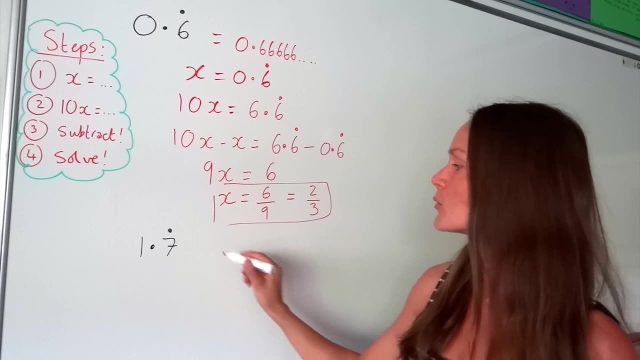 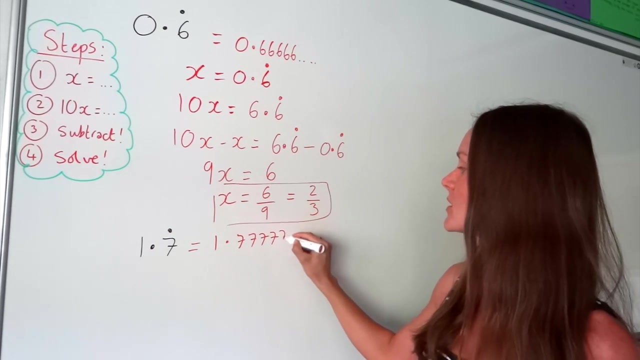 So 0.6 recurring, when we write it as a fraction, is the same as 2 over 3.. OK, so I'm going to do exactly the same thing for the next one. So just remember that the dot is above the 7.. So this number is the same as 1.777, with those 7s never-ending. 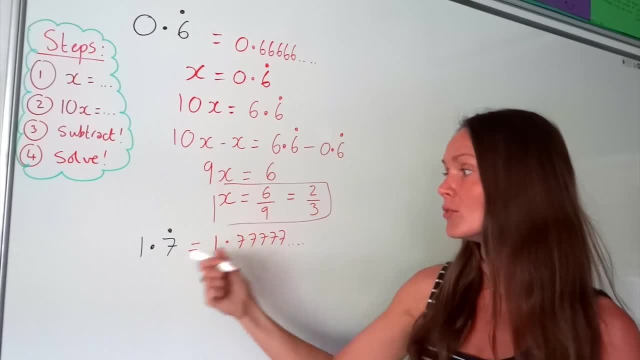 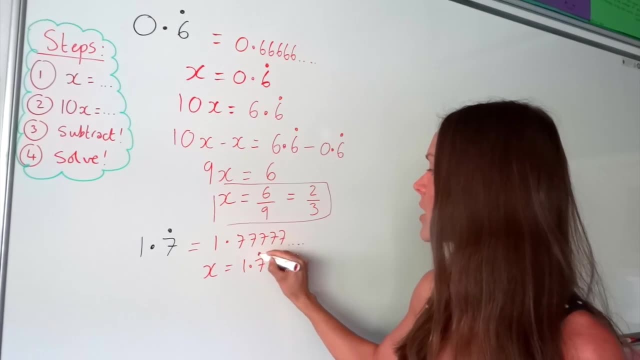 So remember, step number 1 is to put our original number equal to the letter x. So I'm going to write: x equals 1.7 with the dot. Then step number 2 is to calculate 10x, So I'm going. 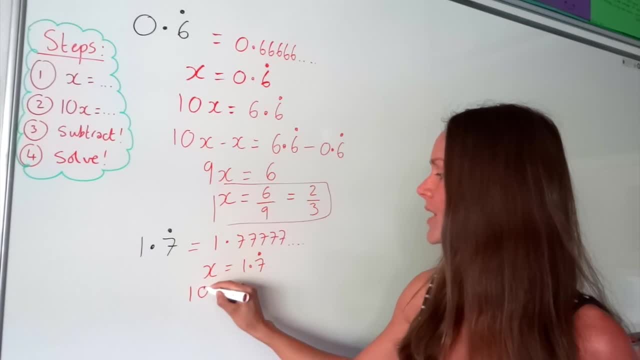 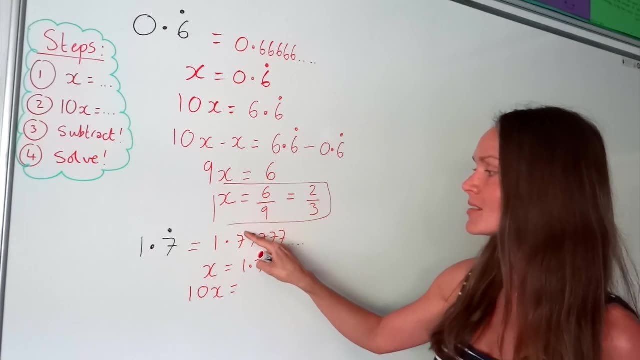 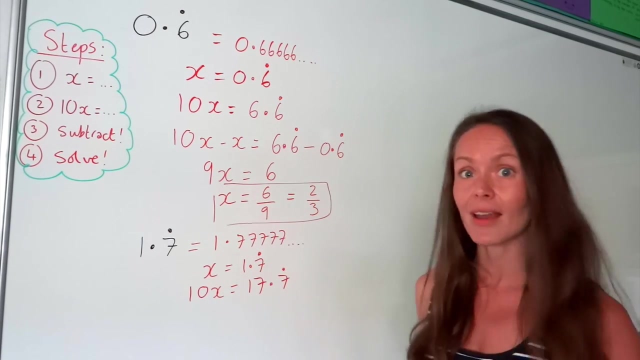 to write 10x. So I'm multiplying x by 10 on the left, which means I have to multiply this number by 10 as well. So the decimal moves one place to the right. So I'm left with 17.777, which is 7, recurring like that. So step number 3, just like before, we have 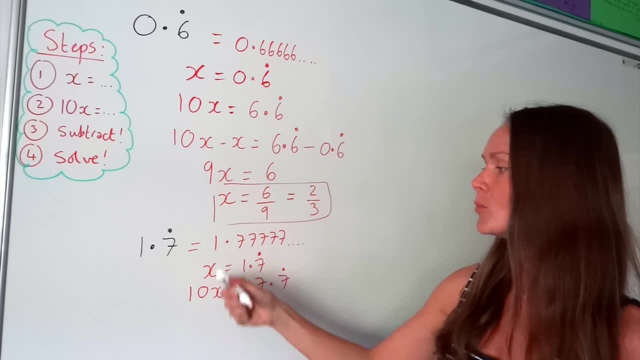 to subtract. So you're doing the larger x minus the smaller x. So we've got 10x minus 1x. So we're doing this larger number here: 17.7 recurring minus the original number 1.7. 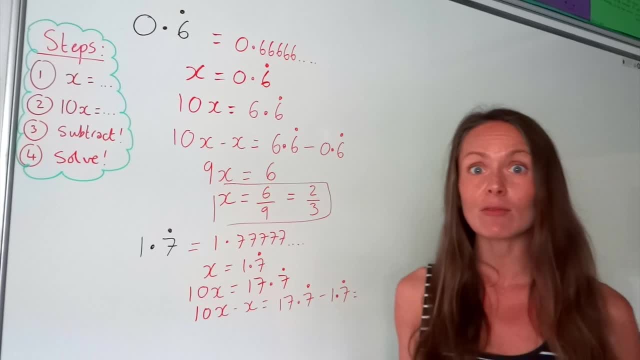 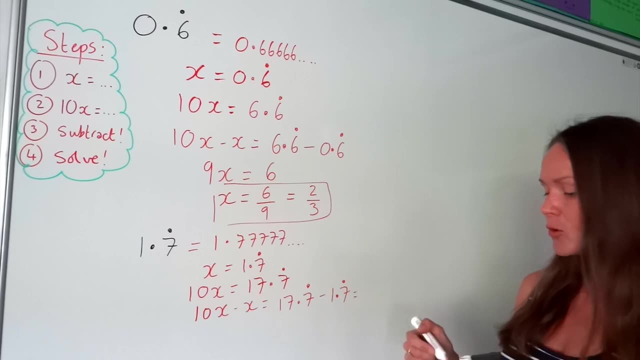 recurring. Now, remember, we're doing this to get rid of those recurring decimals. If we do 17.7 recurring minus 1.7 recurring, well you can see we're automatically getting rid of those parts. But we're also doing 17 minus 1, which leaves me with 16.. 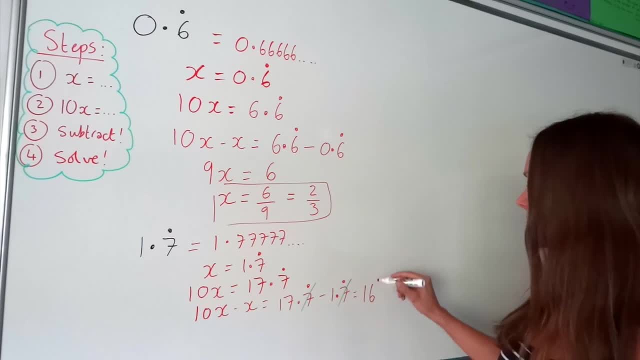 So 10x minus 1x, well, that's 9x again- I'm going to carry on up here- And that 9x is equal to 16.. So the final step is to solve the equation to find x, Because x is being multiplied by. 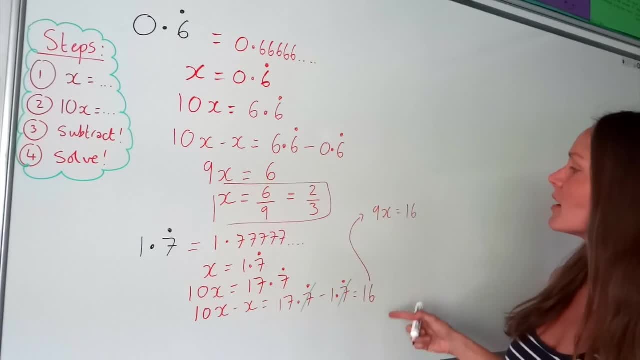 9,. the opposite is to divide by 9.. So we divide by 9 on both sides of the equation. So I'm left with x equals 16 over 9.. And we can't simplify this fraction. So there we go, OK. 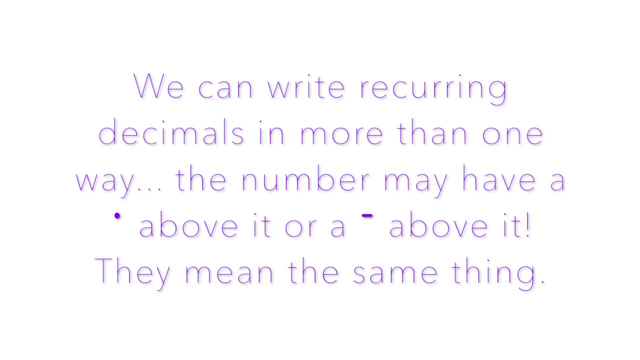 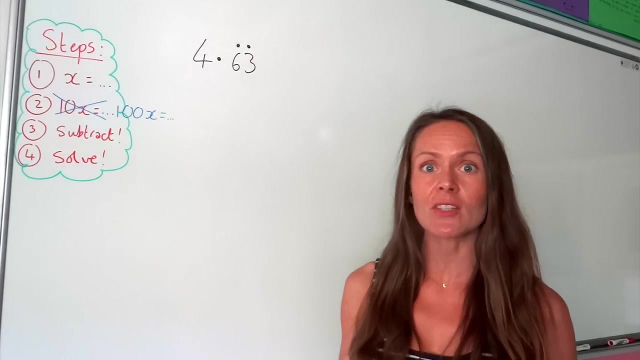 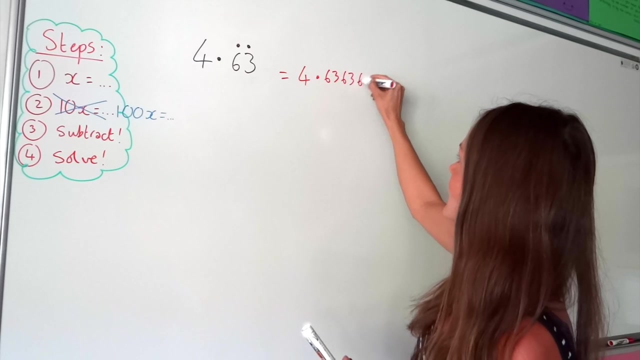 let's try it, Let's do it a little bit harder. OK, so this time it's a little bit different, because we have two numbers repeating after the decimal instead. So we've got 4.636363.. So we've got both of those numbers repeating. Instead of just having one repeating, we're going to do a little bit harder. So we've got 4.636363.. OK, so now we're going to try this again. So this is our number that we've got here: 6.636363.. 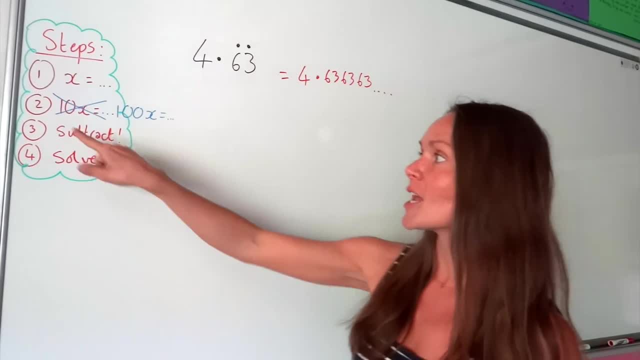 So we've got 4.636363.. OK, so now we have 2, 6.636363.. So we've got 4.636363.. like in the previous two examples. So that means step number two is going to change. 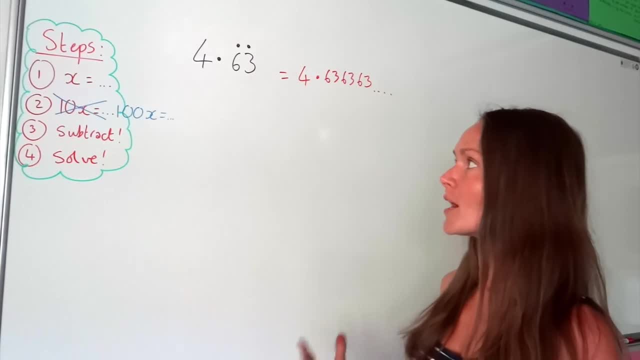 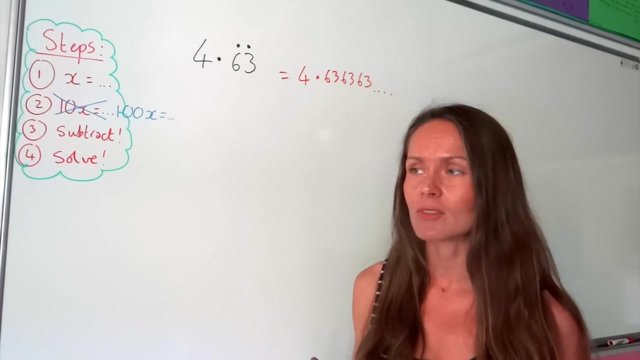 Instead of calculating 10x in step number two, we now calculate 100x, because there are two numbers after the decimal that are repeating. We want to multiply by 100, so the decimal moves two places. to get rid of those recurring decimals, Well, let's have a go. So I write my x equals to start. 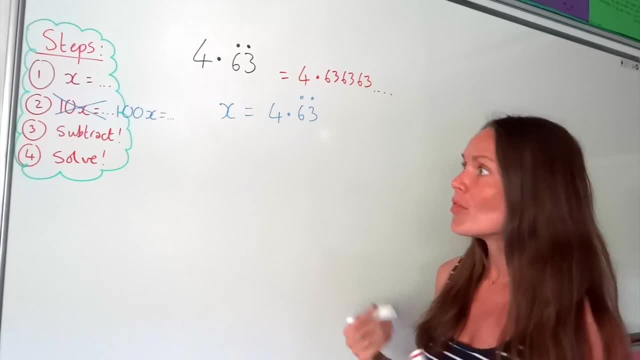 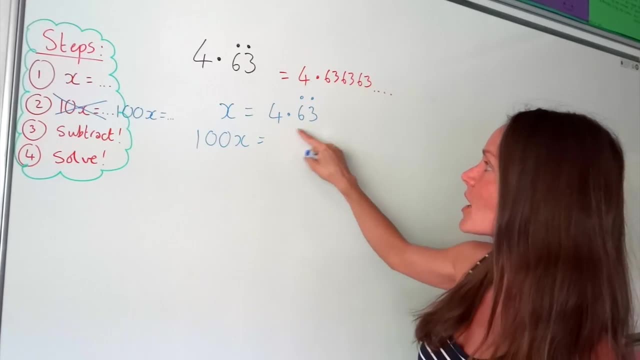 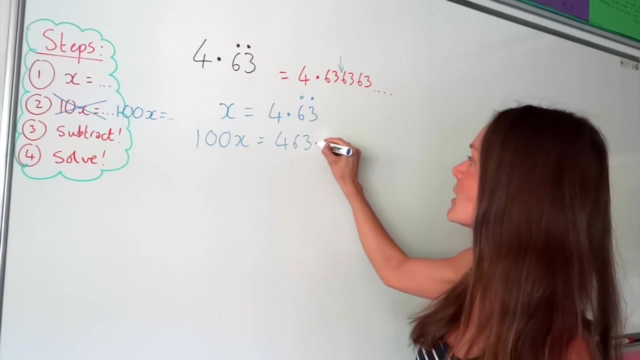 with, So it's equal to the original value. Then I have to work out 100x, So multiply both sides by 100.. So if I times this by 100, the decimal moves two places to the right. So I'm left with 463.63. 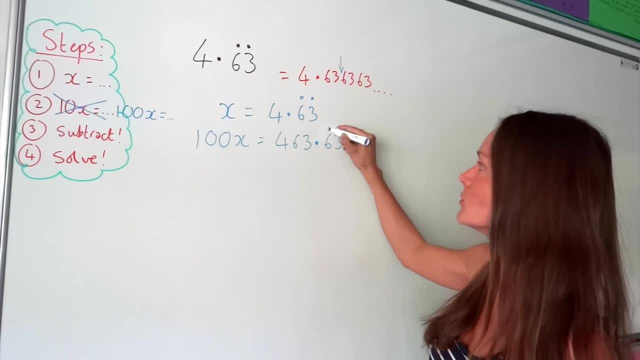 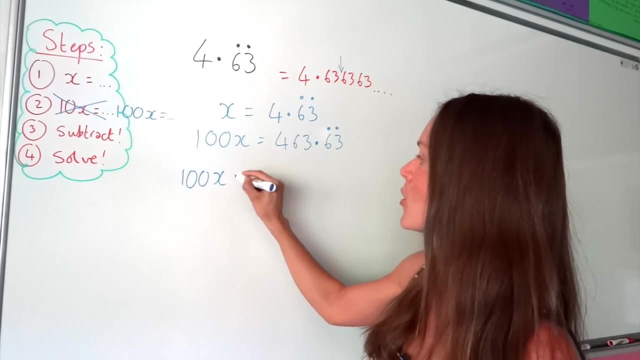 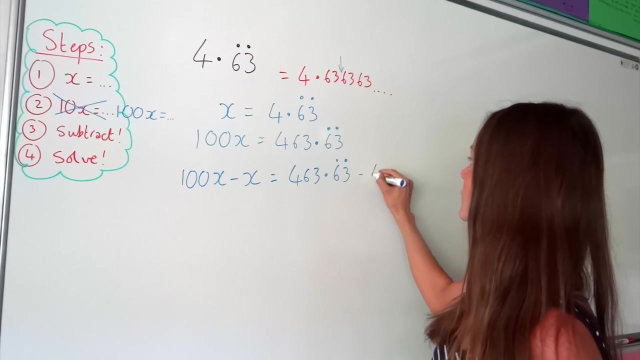 recurring, because those numbers are still repeating. after that new decimal, Now step number three. just like before, we have to subtract. So you're doing 100x minus 1x, So the bigger number here minus our original value, And then we can work this out: So 100x. 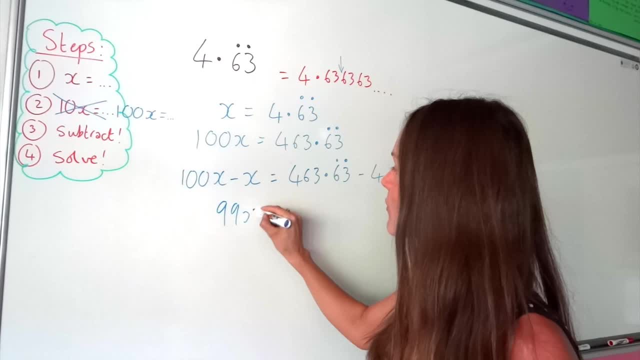 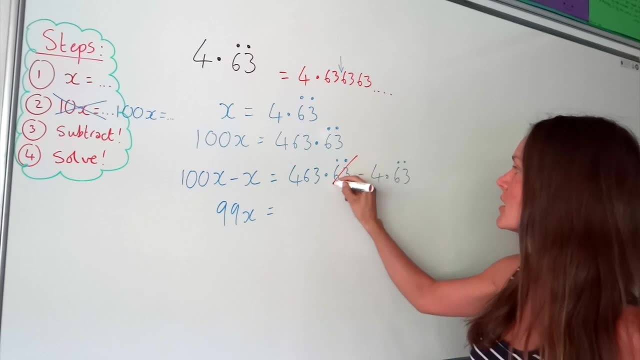 minus 1x is 99x On the right-hand side. well, when I subtract these, I've got the 0.63 recurring minus the 0.63 recurring, So we've managed to get rid of our recurring decimal here. 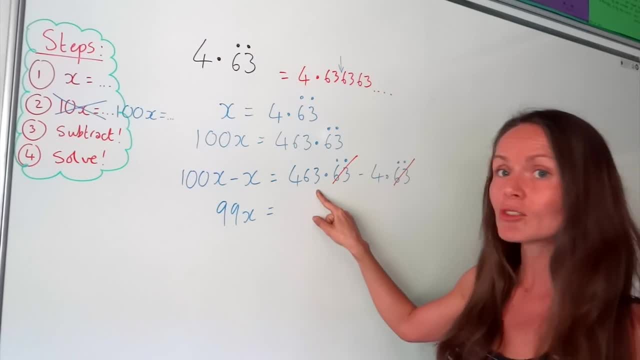 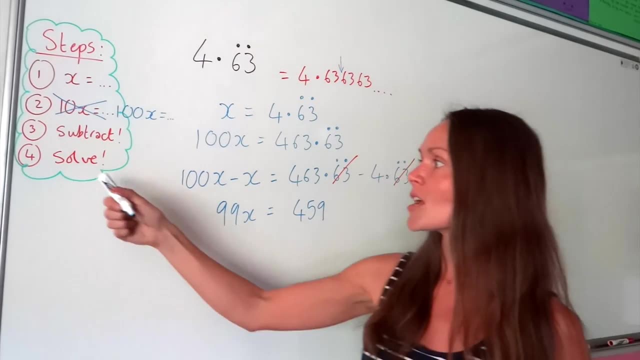 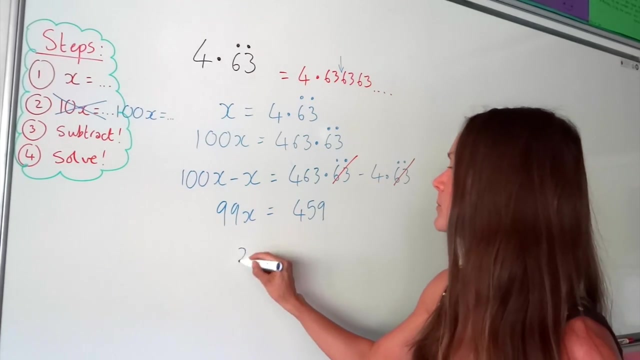 Then we have to subtract these numbers as well, So 463.63.. Takeaway four is 459.. So the last step, step number four, is to solve the equation. So I need to divide by 99 on both sides of the equation. So here's my fraction, Although I can simplify. 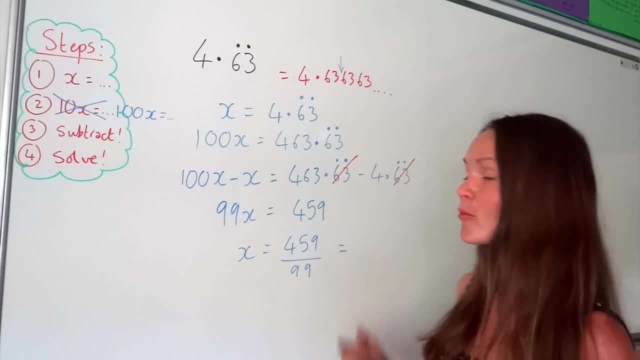 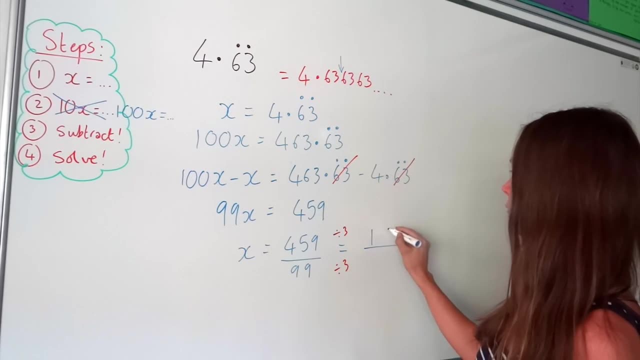 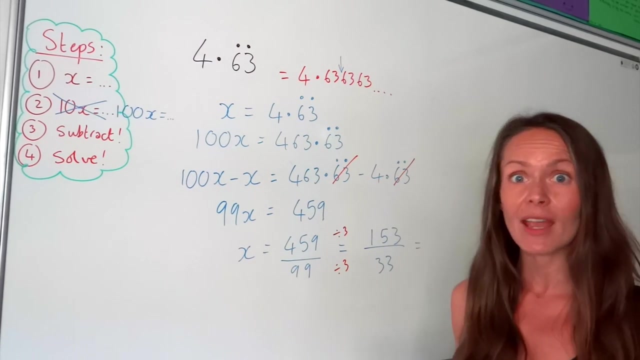 this fraction, I can divide both the numerator and the denominator by three. So when I do that, on the top I now have 163.63.. 153.. And underneath I have 33.. And I can actually divide that by 3. again, 3 is a common. 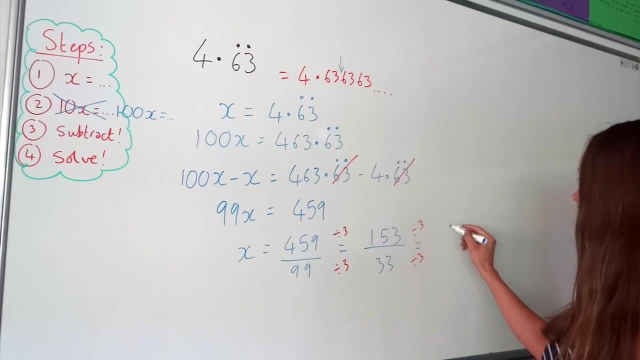 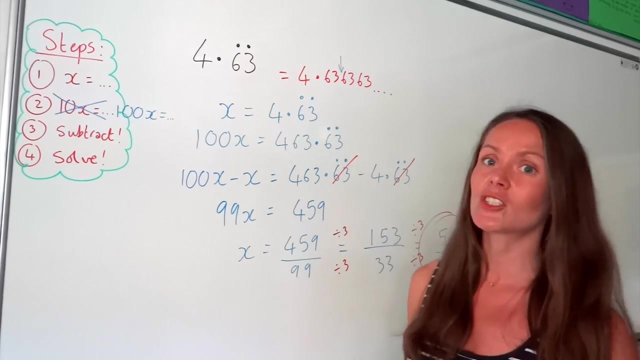 factor in both the numerator and the denominator. So that leaves me with 51 over 11.. So that's the final fraction in its simplified, final version. So there you go. I've got one more example to finish where we have more than two repeating numbers after the decimal. 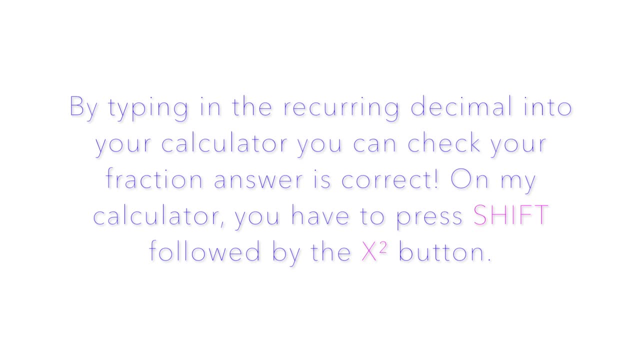 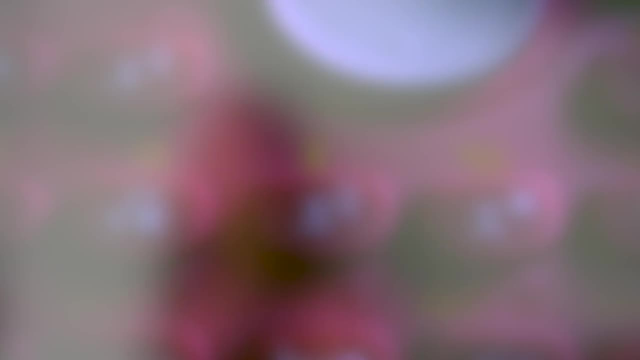 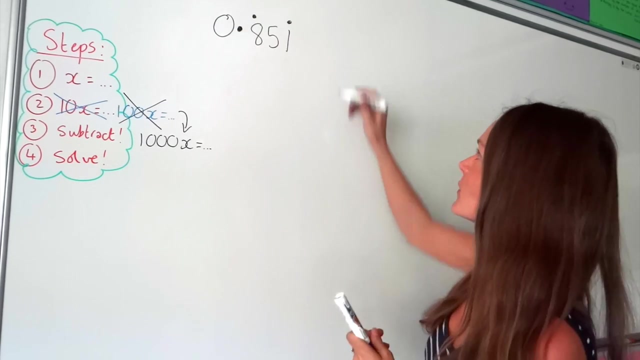 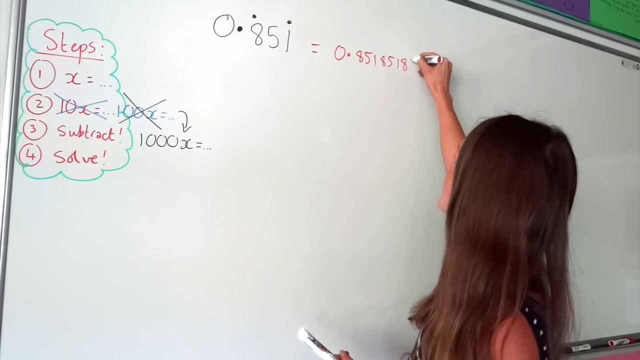 OK, so in this last example we now have three numbers that are repeating after the decimal point. So this number up here looks like this: It's 0.851,, 851,, 851, and so on. OK, so they. 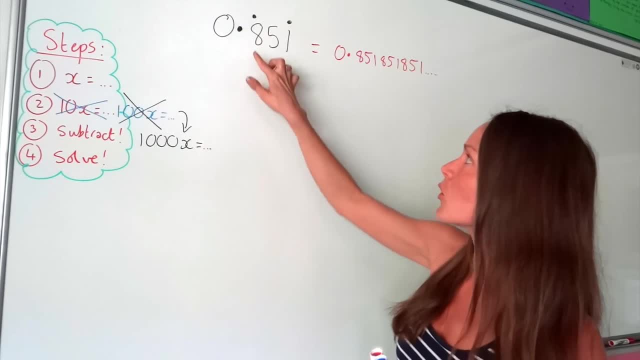 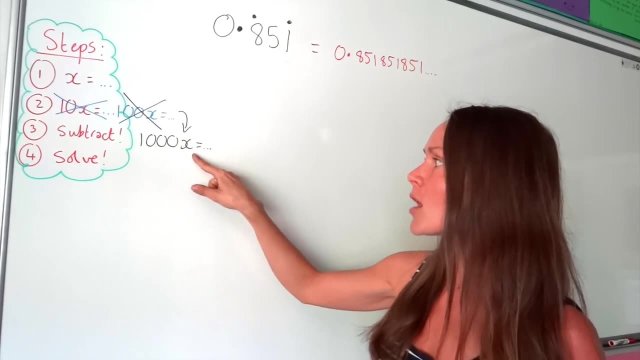 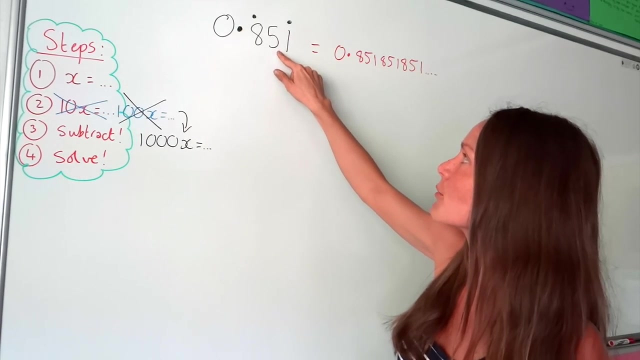 keep repeating themselves. So we need to try and get rid of the number that's repeating after the decimal point. So step number two is now multiplying x by 1,000. Because if we multiply by 1,000, the decimal point moves three places to the right. So we can get rid. 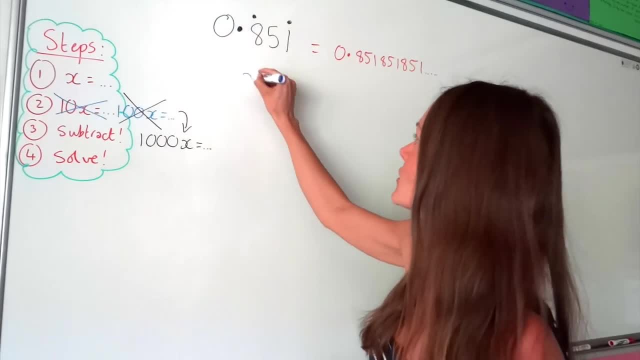 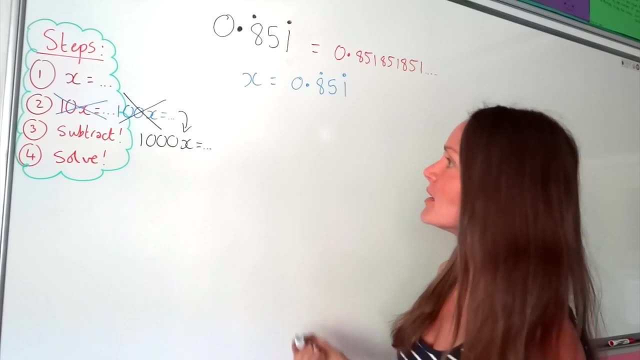 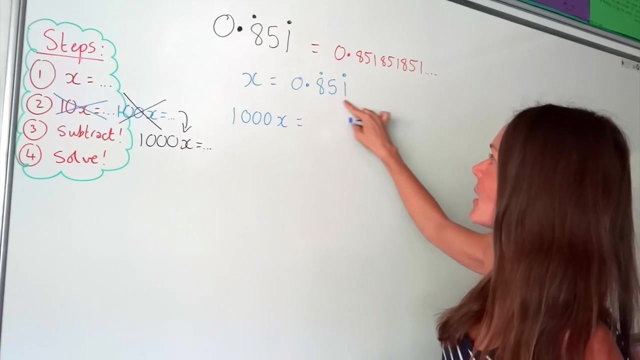 of those repeating numbers. So let's have a go. So, just as before, we start by writing: x equals with our original number. Then step number two, this time is to calculate 1,000 x. So if I multiply this number by 1,000, the decimal moves three places to the right. 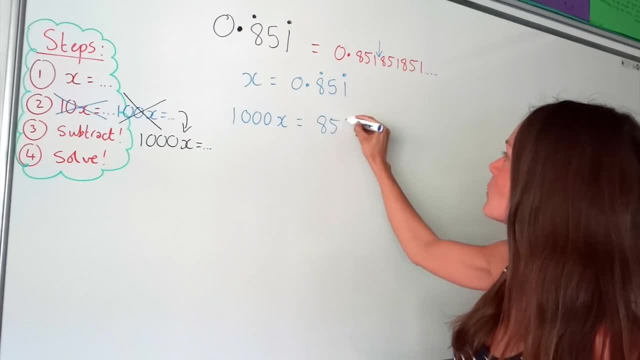 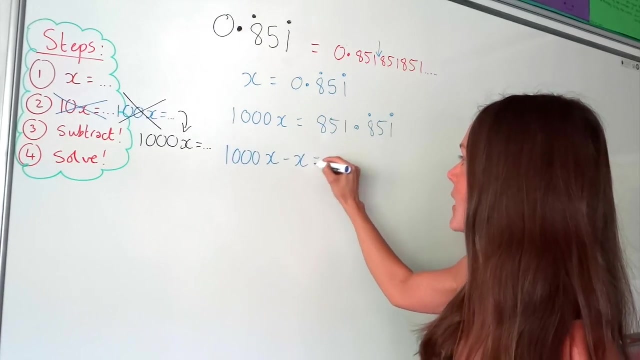 So it goes to here. So we're left with 851.851 recurring. So those numbers after the point are still recurring. OK, Now step number three. just like before, we have to subtract. So you're doing 1,000 x minus that single x value. So we've got the big number minus. 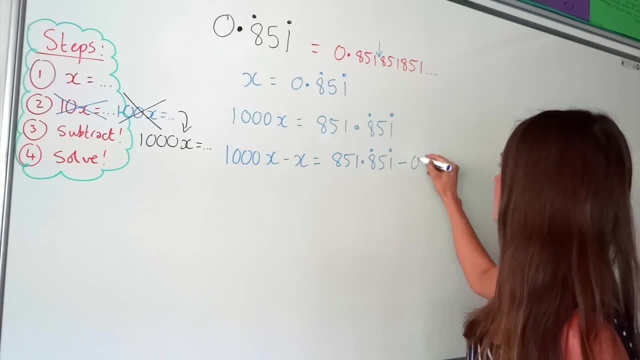 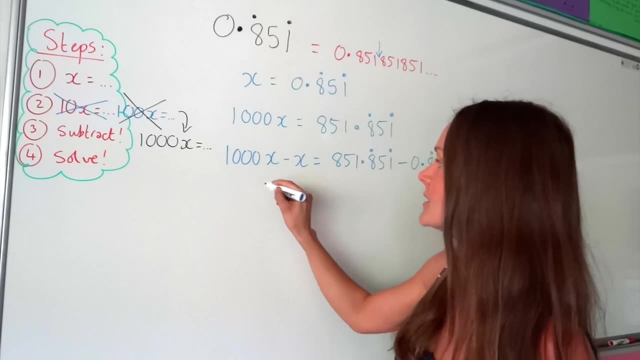 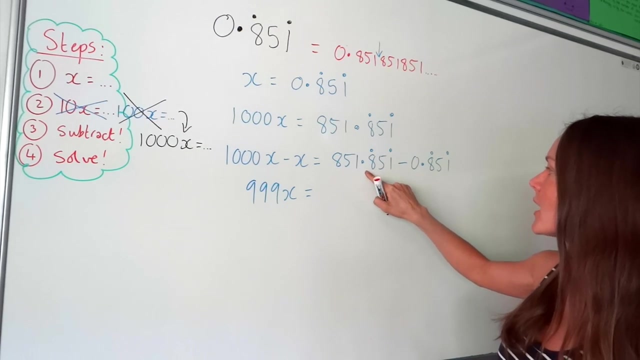 the value of 1,000.. And now we can subtract. So 1,000 x minus 1 x is 999 x On the right-hand side. if I subtract these numbers, well, I've got a 0.851 repeating minus another 0.851 repeating. 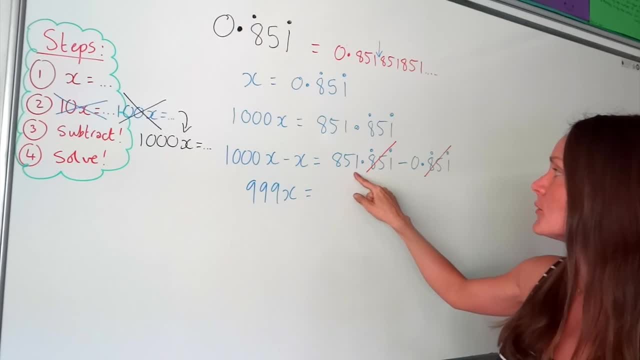 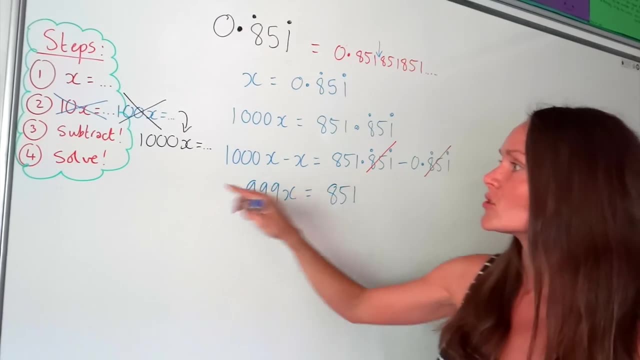 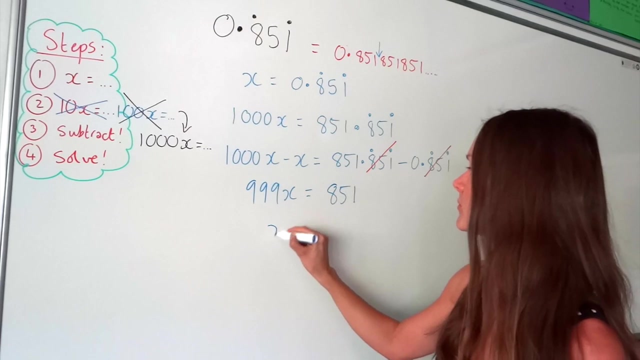 So they go to 0.. And then I've got 851. take away 0.. So I'm just left with 851.. So the final step is to solve the equation. So I need to divide both sides of the equation by 999.. So I'm left with this fraction. OK, This fraction. it does simplify, It's quite. 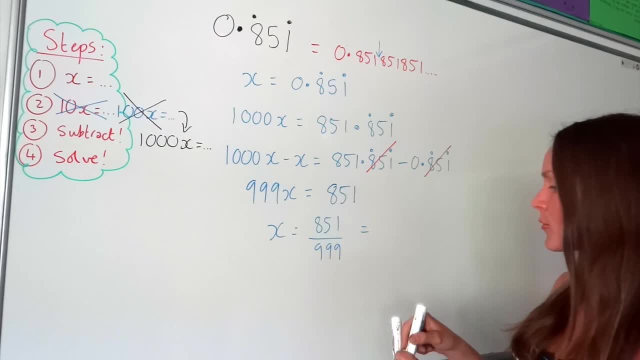 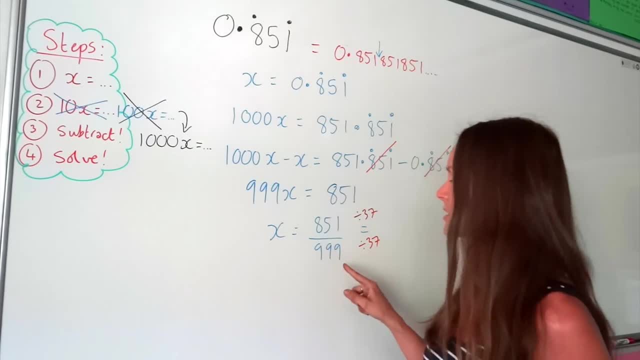 thing. You're going to get the same thing. You're going to get the same thing. Just remember that when you look at this on your calculator, your calculator should give you the simplified fraction. OK, So you could cheat a little bit on that last step. 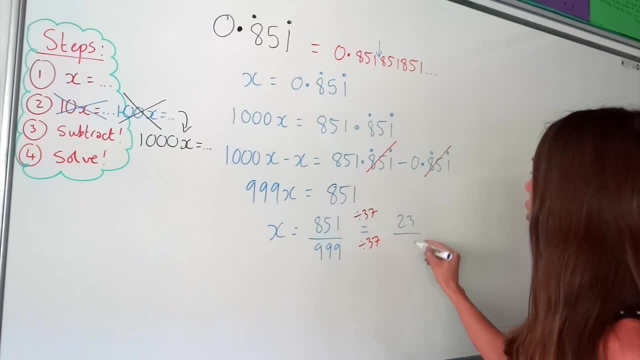 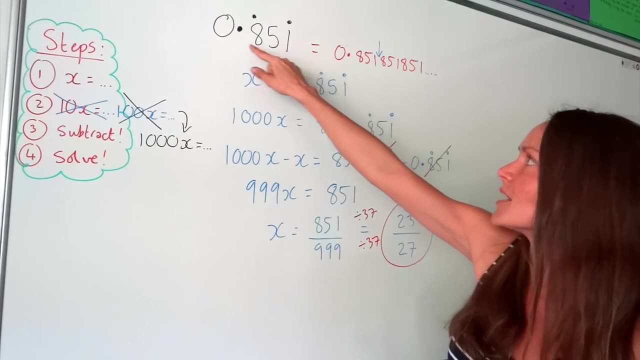 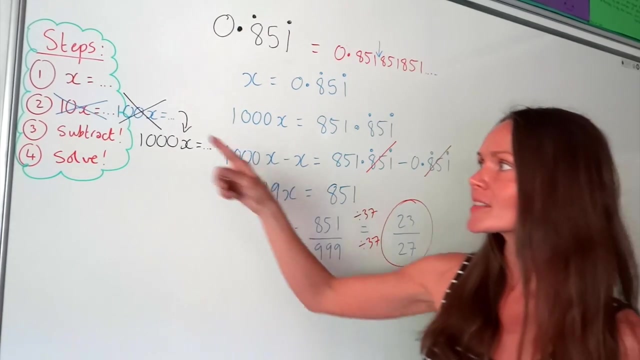 So when we divide those by 37, we get 23 over 27.. OK, So there's the final answer. OK, so this repeating decimal is written as 23 over 27.. OK, so I hope that makes sense. now, Just remember: step number two can change If you've got. 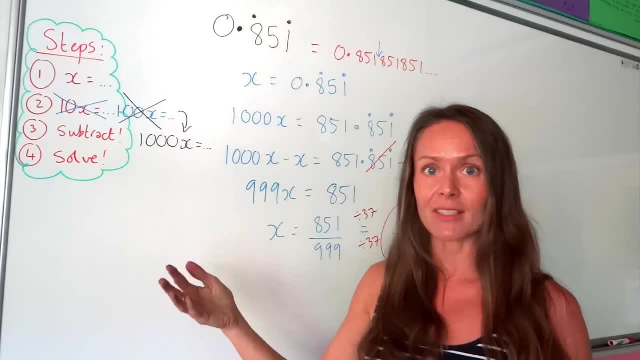 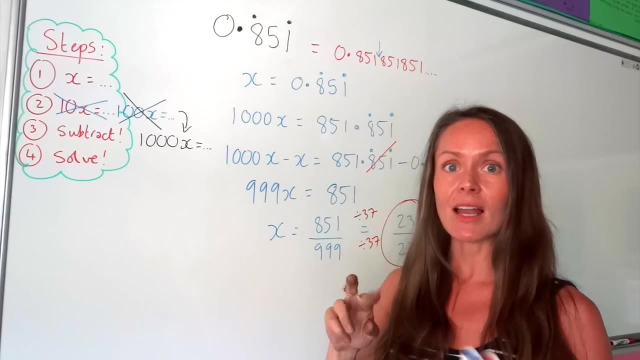 one single number that's repeating, like thisyual number, as you see here, then count it in those heart beaters at 0.3333, you are just finding 10x If you've got two numbers that keep repeating. 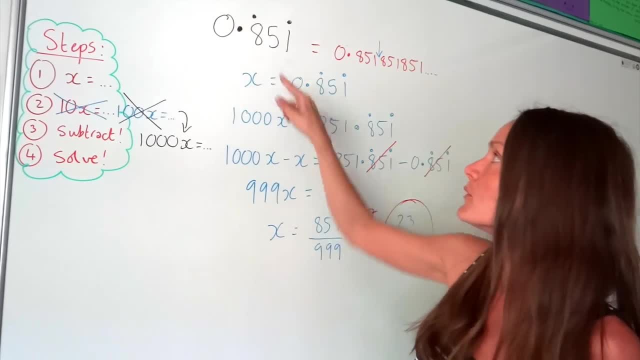 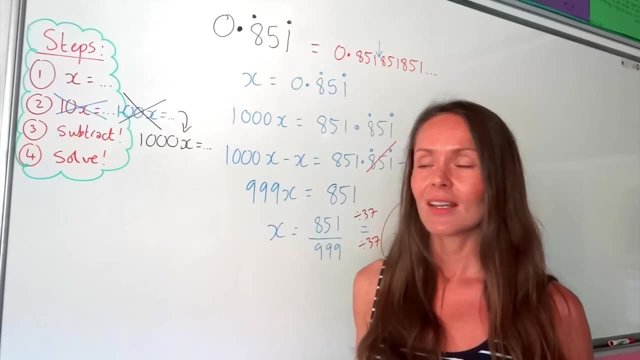 like 282828,, you would work out 100x, And if you've got three numbers repeating, like this one, you would work out 1000x, and so on. But all the other steps are the same And just remember to simplify your fraction where possible. 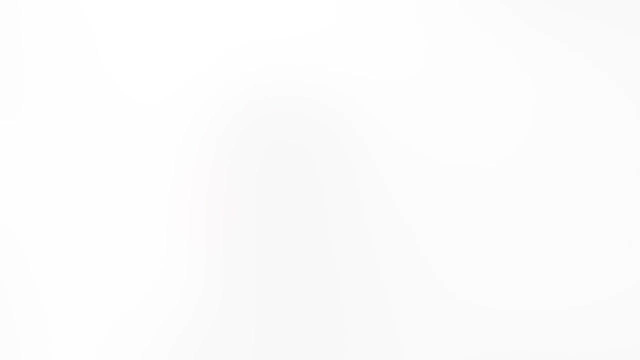 Okay, so that's all from me for today and goodbye.